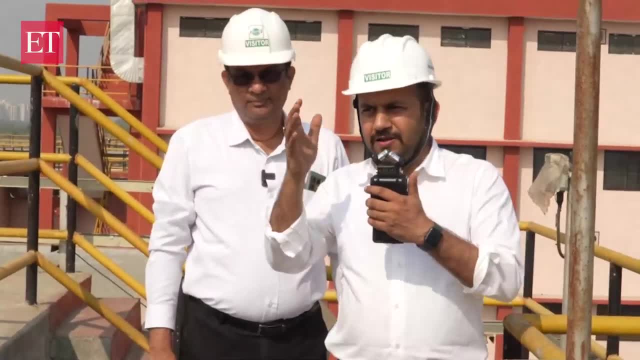 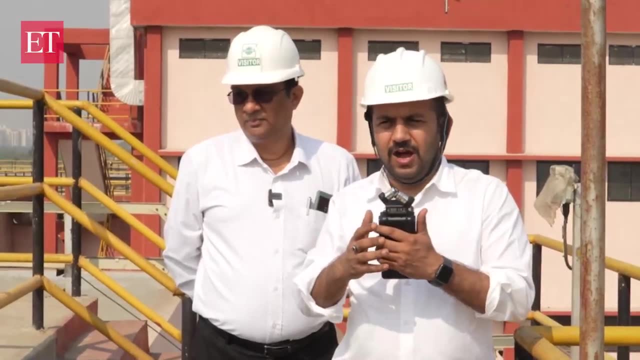 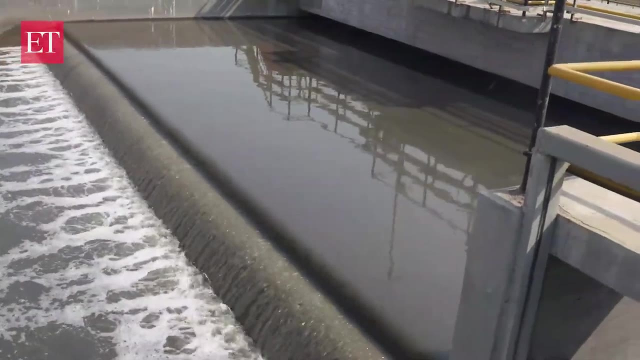 So once that sewage comes to that chamber inlet chamber it goes through mechanical screening where all the other particles, like plastic materials, are sorted out. Then it comes to something called a grid chamber. The heavy particles that is called grid is also coming with this sewage and in this it will be settled and the sewage will be reused. 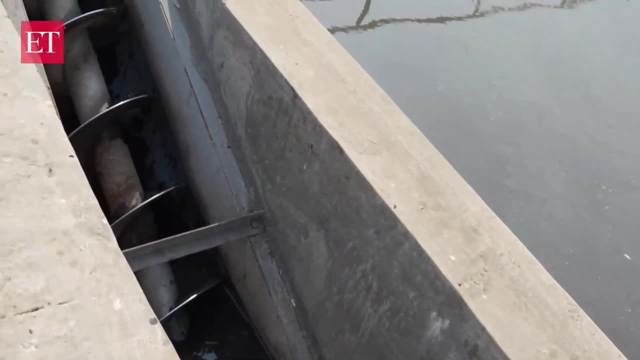 So this is the process of milking, and the treatment of the sewage is here. This is the process of milking, and the treatment of the sewage is here. So this is the process of milking and and with this screw mechanism, it will be separated out and taken out. 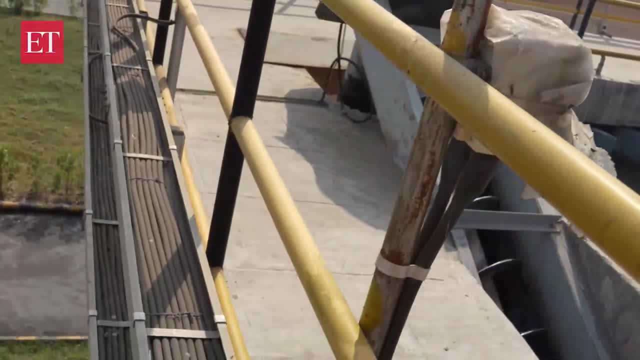 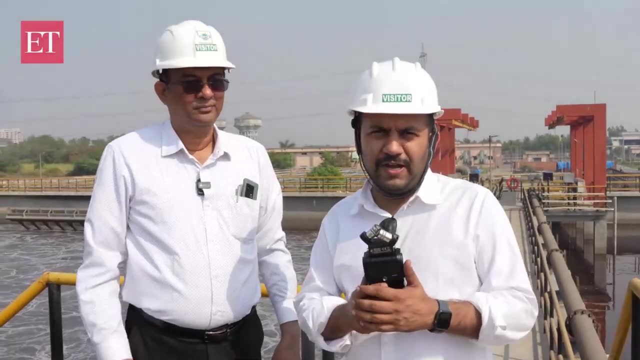 It is separated and you can see at the bottom it is being collected and through this tractor we are disposing to this Khajur disposal plant. So once the process of separation of grit takes place, the water comes to the different chambers, and here there are three processes involved. 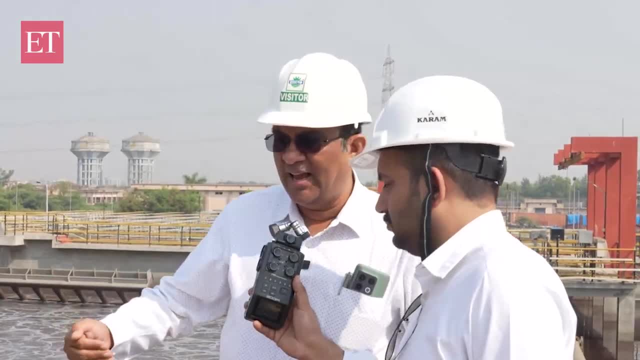 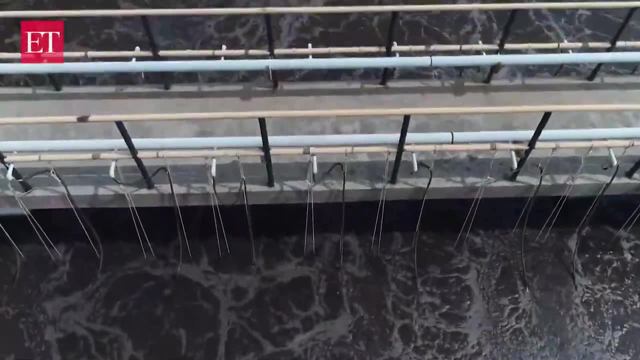 In these three processes, whatever one is filling, and you can see here: first the aeration will be provided, After the aeration, this will be settled in this. So this is stagnant water and in that last is a decanting, the water will be taken out. 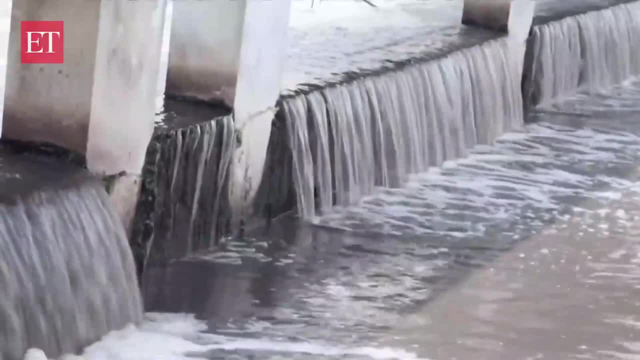 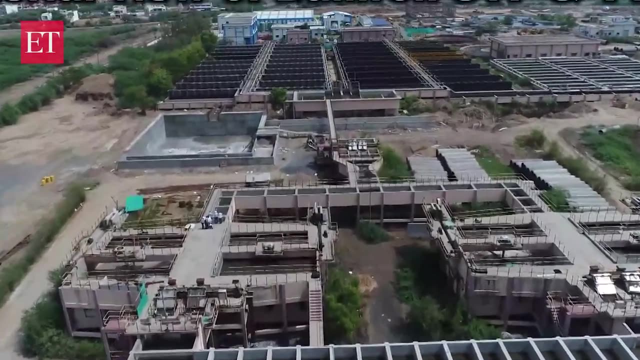 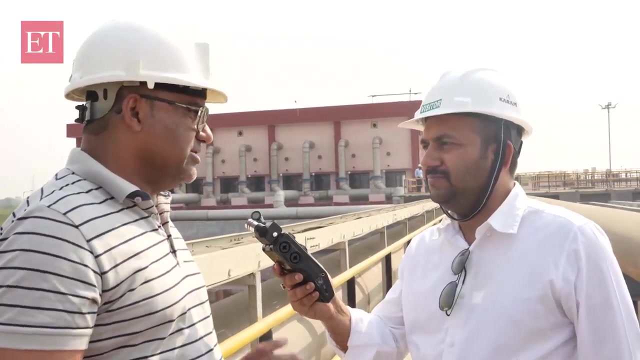 All entire biological process takes place in one single chamber instead of different chamber. That's the reason how you can save the space. My name is Priyash Magajwala. I am the plant in charge here. This treatment facility is called sequential batch reactor technology. 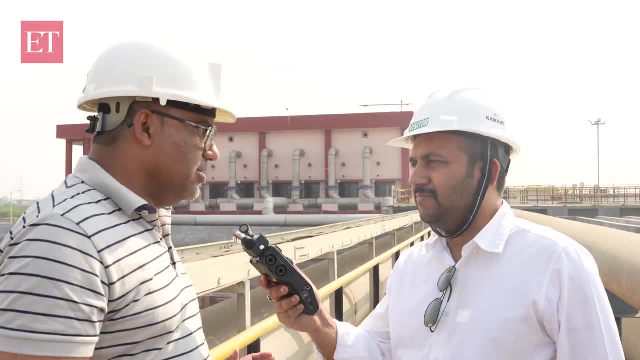 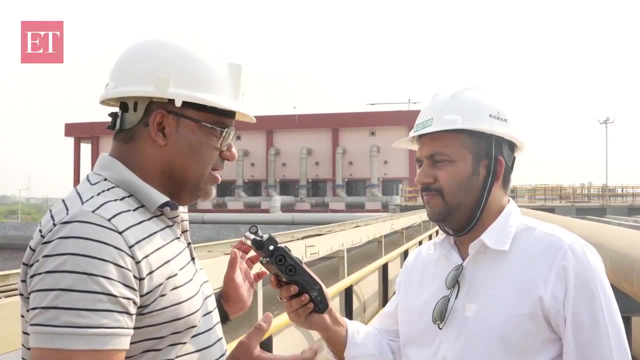 Here we have a system of sequential batch reactor technology. The air in this is a biological process. In biological process we have to maintain the food micron ratio or FM ratio. So the purpose of giving air in this is that the bacteria which are there biologically 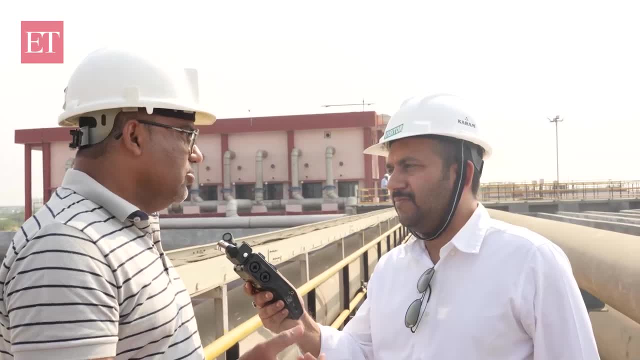 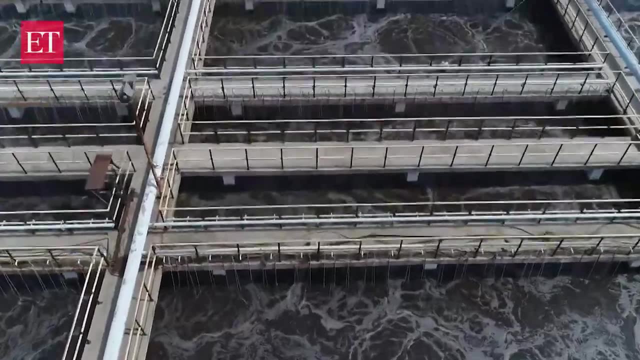 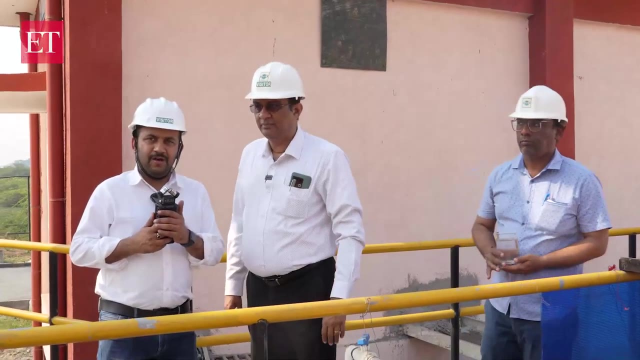 to keep them alive, you have to give oxygen from outside, So for this we give them air, due to which those bacteria remain alive, and the bacteria eat the sludge in the sewage water and the food. Now we have come to the UV chamber. here ultraviolet rays are going to be used to kill the bacterias over here. 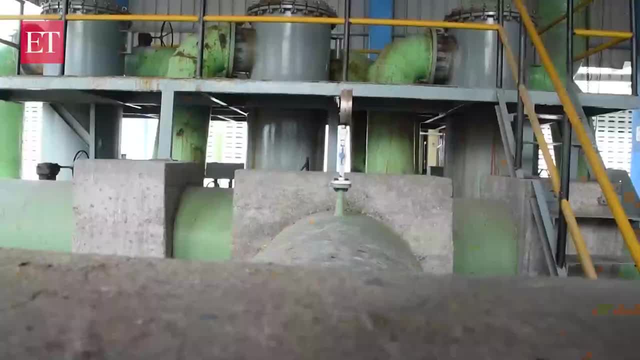 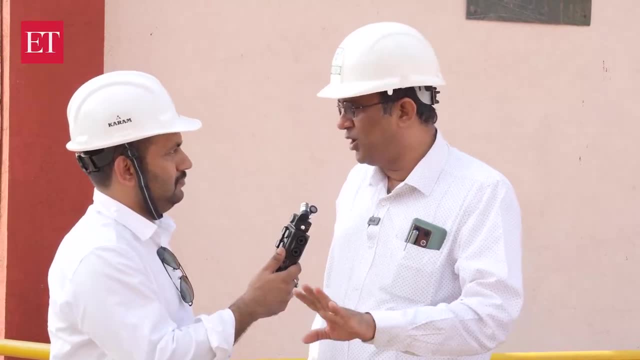 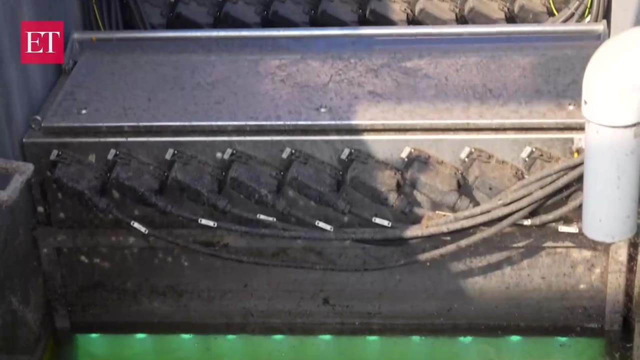 Poly form bacterias, so that nothing will remain in this All the, whatever the bacteriology, something is left out. it is also cleared here and secondary process is completed at this end. You can see the water is taken out from the UV chamber. 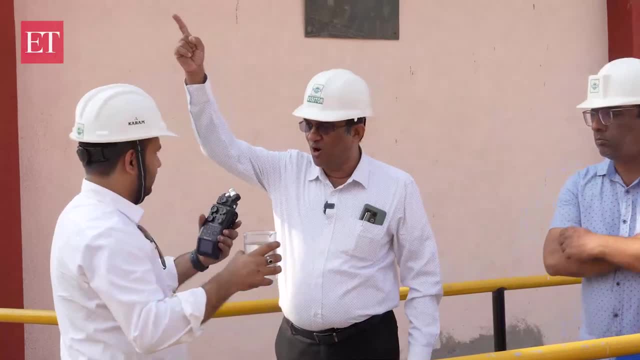 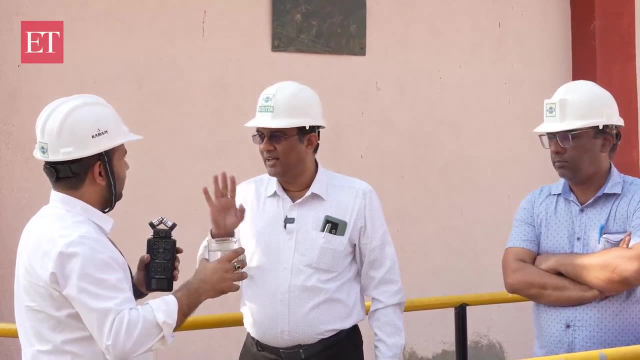 So this is the water. This is the water You saw, the first water there, and now this is the secondary treated water. This can be released into the. This can be released into the river as well as creek. Okay Water course is available because we are treating as per the pollution control board standards. 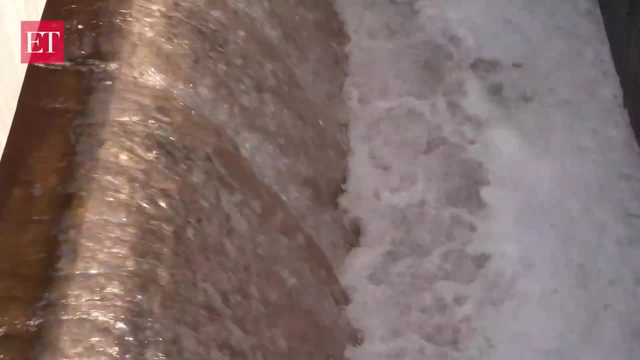 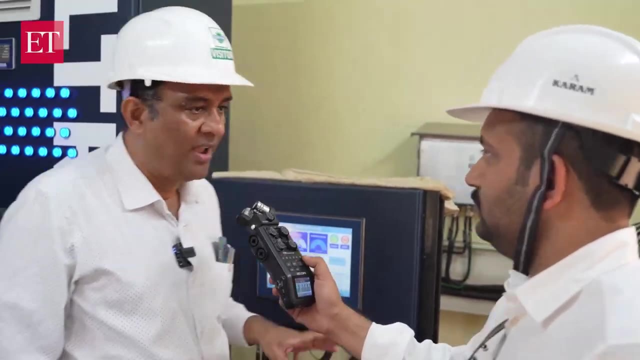 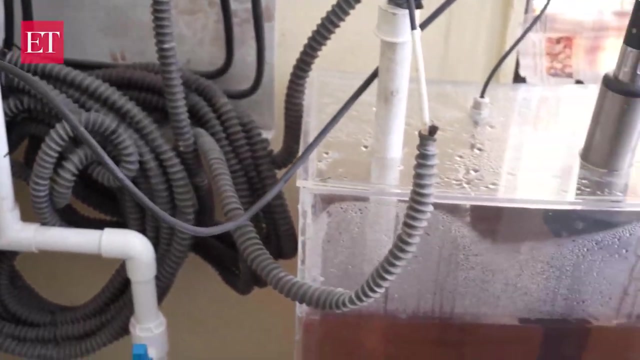 Okay, We are in the UV control room. Whatever the water is being treated, there are certain parameters as per the pollution control board that will be observed online on this And that is connected with the pollution control board. The data is directly fed to their area. 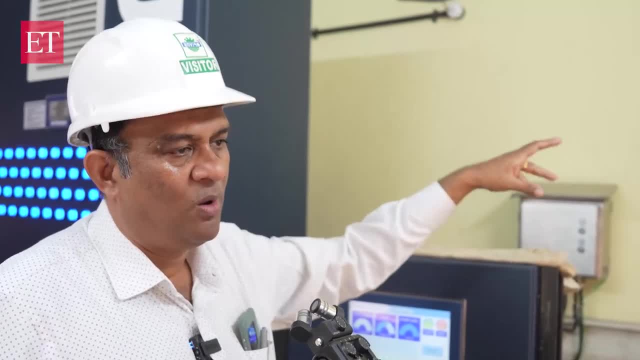 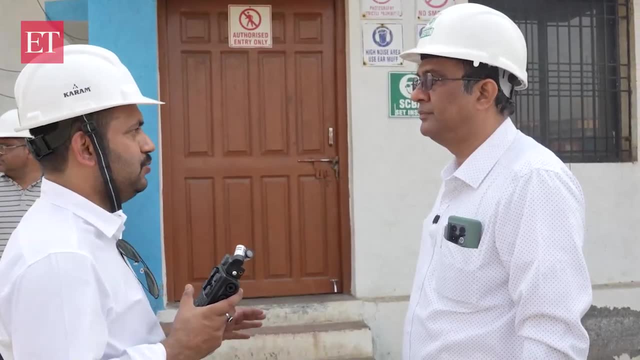 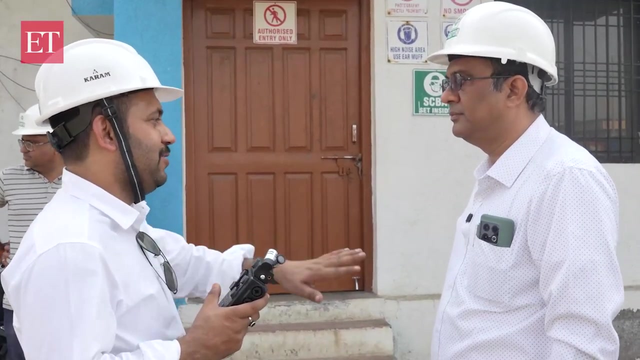 So even pollution control board also can come to know what are the disposal parameters available in this plant. They say there are a lot of energy is used in running this kind of a plant. So don't you think it's like a dichotomy here that you know once you're trying to clean water, the energy is also getting utilized? 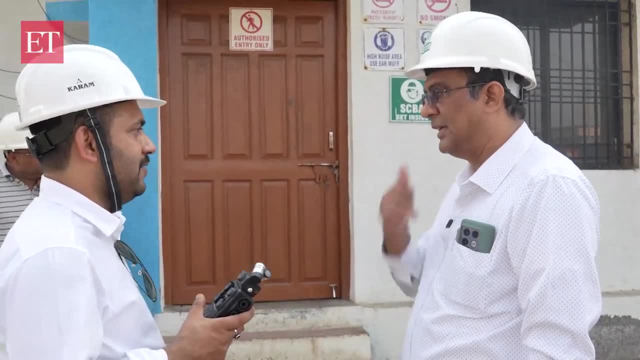 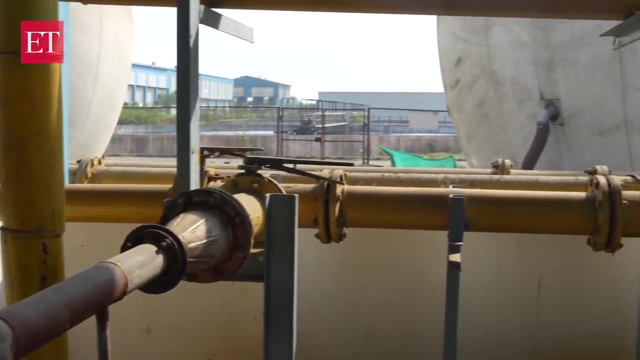 And that energy is coming from somewhere. So what have you done for that? So, as far as the sewage plant is concerned, whatever the sewage gas generated after the due process that is normally to be flared up. from this, you can see that that is the flare provided. 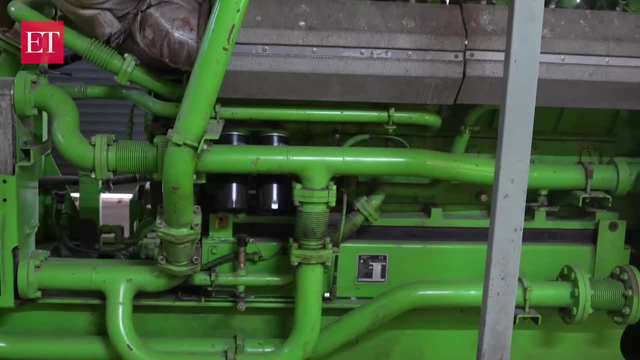 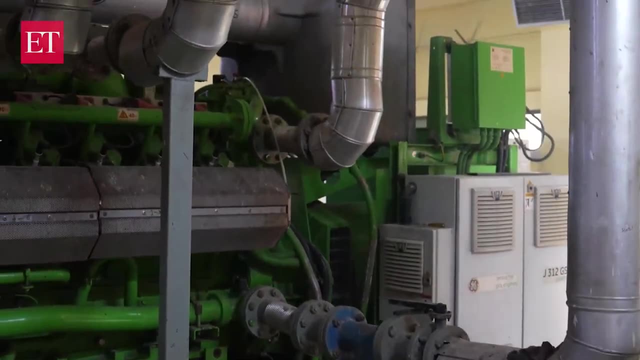 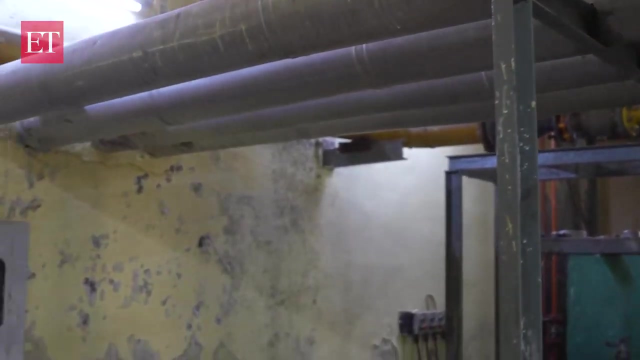 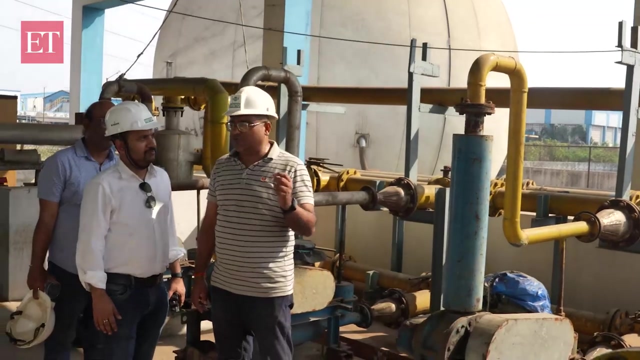 Now we what we did, that we have provided gas engine into it. We are using that first into that gas. We are That gas is going to scrubber where that 2S is removed And whatever the pure methane is extracted From there that we are feeding into our gas engine, and from this gas engine electricity is generated that will, you know, provide around 30 to 40% electricity demand of the plant itself. 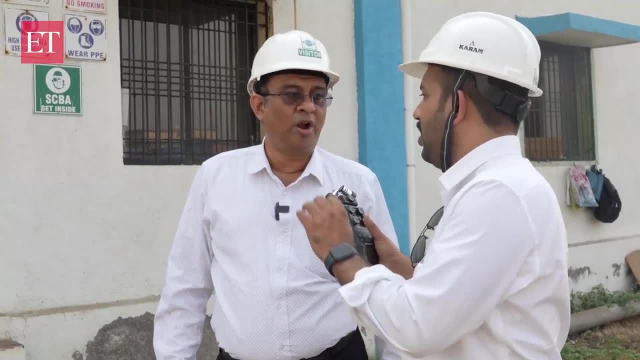 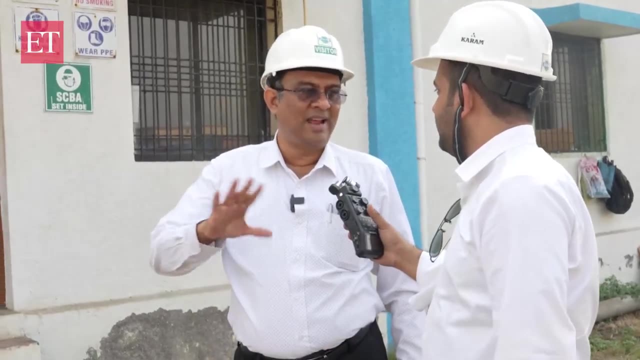 Three megawatt is the total demand and five megawatt 0.5 megawatt. 0.5 megawatt is what you kind of generate from the Generate from a plant that is around 10% right now, but it will increase up to 30%. 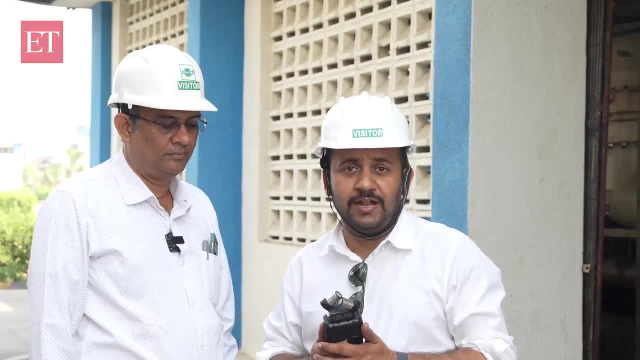 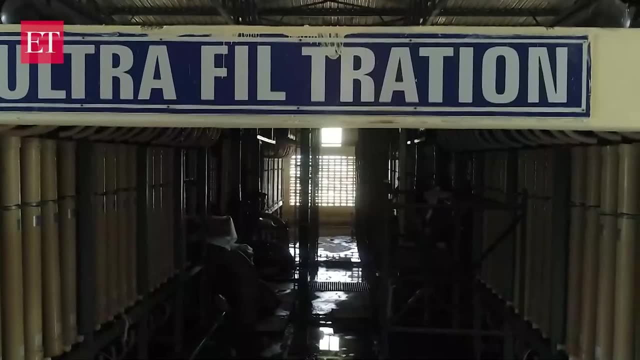 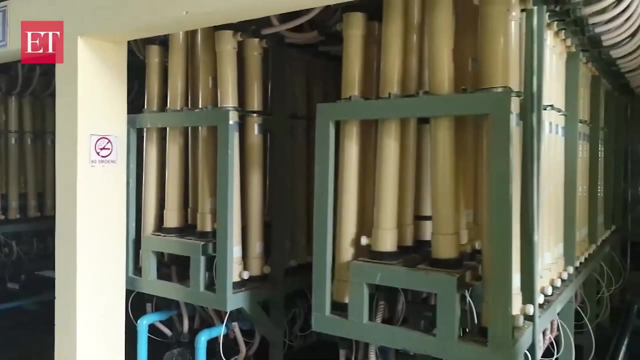 In the third process, Where the tertiary filtration started, We went to the disc filter. Once the water goes to the disc filter, it then comes to UF and RO, ultra filtration and reverse osmosis, And the water that we saw at the start of the video will look something like this: